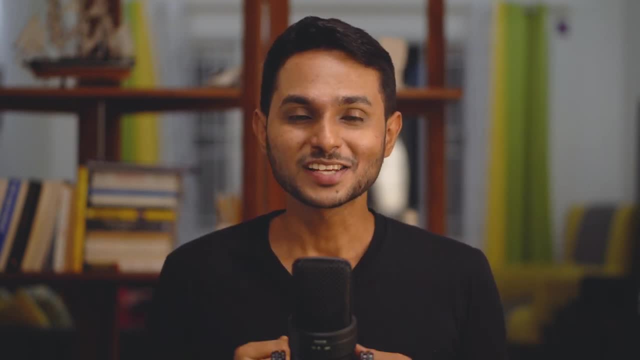 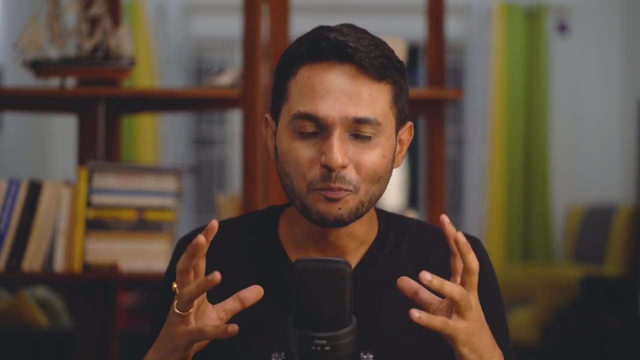 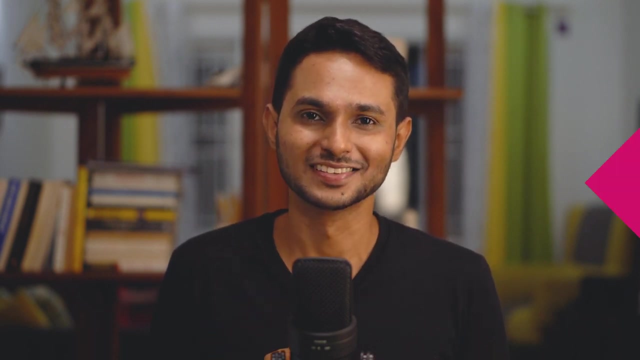 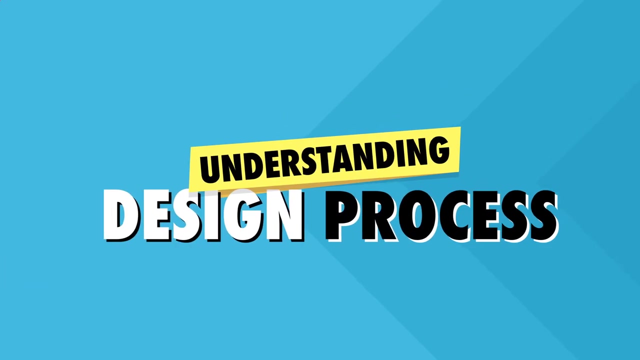 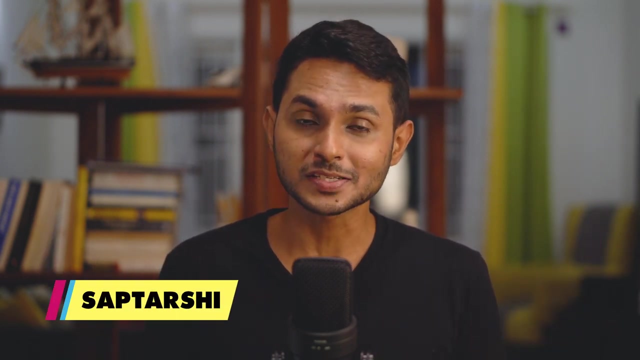 of new things and solutions. This magical box is called design process. Let's try and find out what this magical box is all about and what is the most important thing in any design process. Stay tuned. Hey you awesome people, Welcome to my channel. This is Saptar, and if you're here for the first, 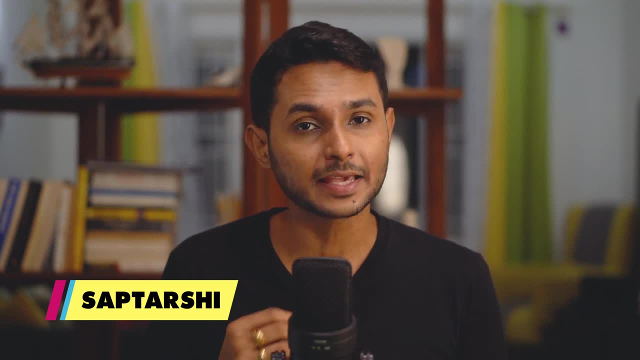 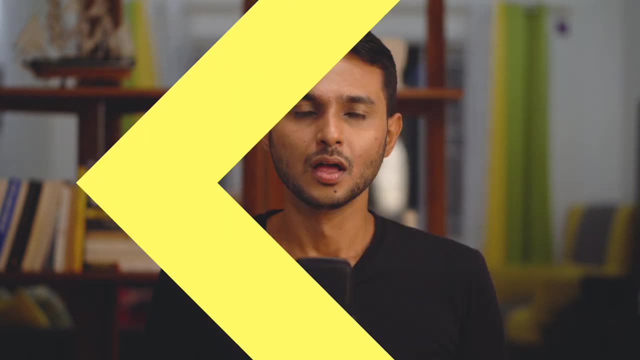 time. this is the place where I help designers build and scale their career with tips, strategies and tutorials, So if you're into it, don't forget to hit the subscribe button. One of the most commonly asked questions to any designer, be it in an interview or 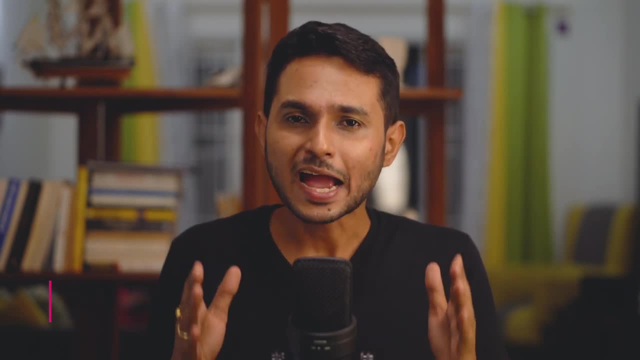 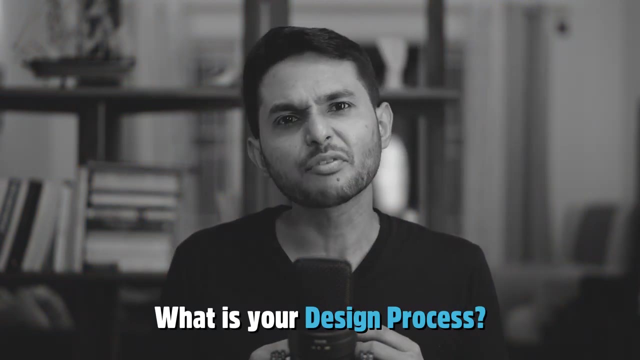 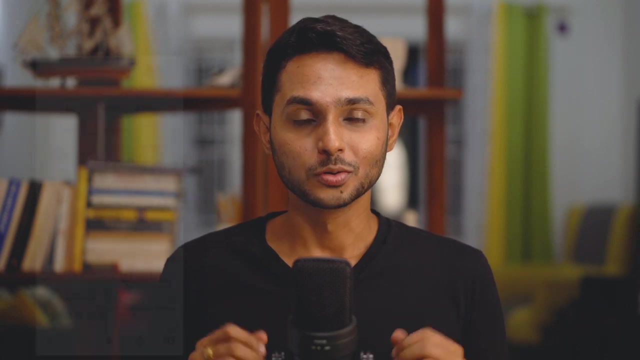 any other forum is: what is your design process? And to that many of us go like research, wireframes, sticky notes. I used to be that guy. When you search design process on Google, you'll find a long list of results with different people. 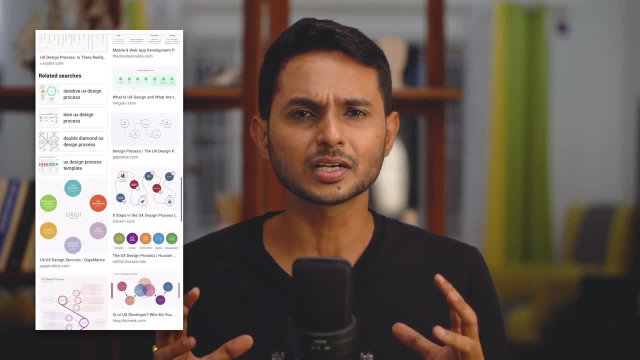 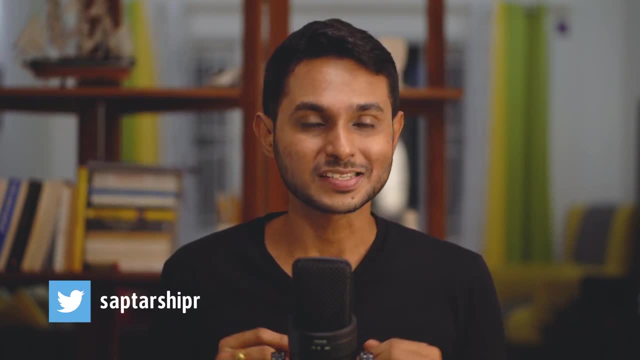 speaking about different steps, things to do, diagrams, flowcharts and a whole lot of things which can get a little overwhelming. So in this video, I'm not going to tell you about my process or somebody else's process. Instead, I will tell you about the core, the most important part, without which no design process is. 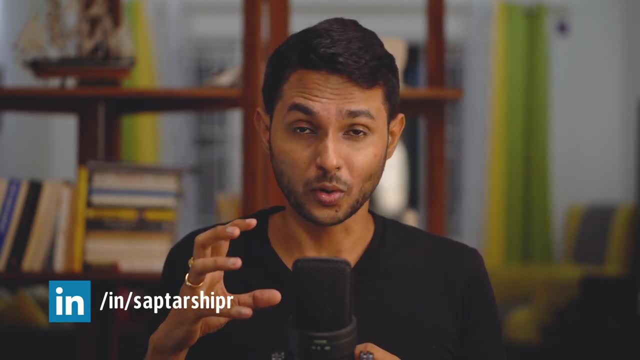 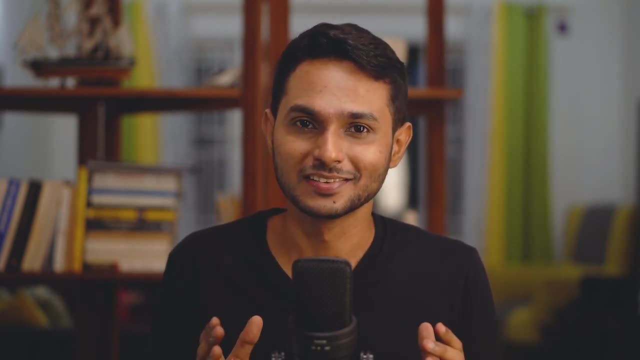 ever complete, So that you can build or adopt a process for yourself which is magical, just because you've done it yourself. So let's get into it. So the first thing you need to do when you're designing a design process is to make sure that 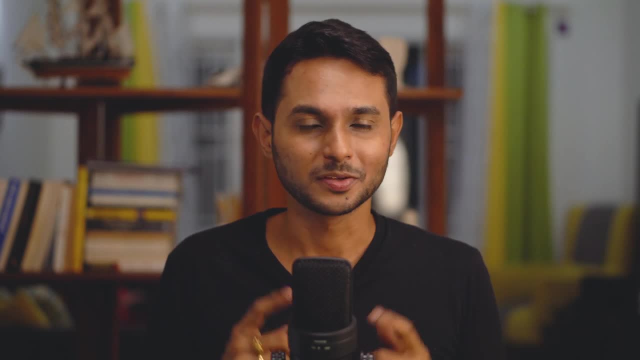 you're designing it for yourself, which is magical, just like the box we had spoken about, Rigid, at the same time flexible. When we design, we often start with an idea and some assumptions around it, where anything can happen. It's like swimming in a sea of infinite possibilities and 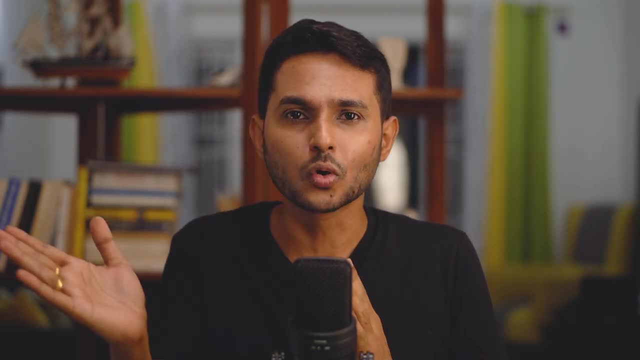 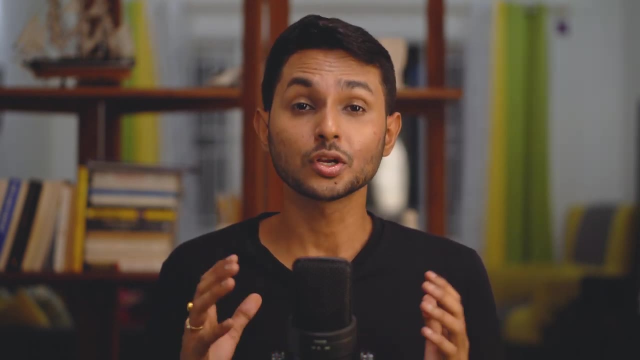 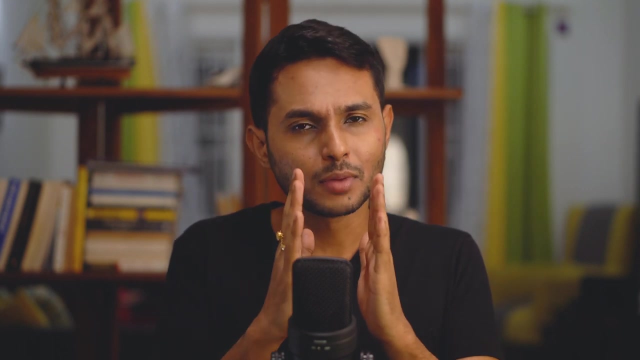 uncertainties, where even a slightest drift can take you around a certain course even before you know. This is exactly where design process comes into the picture. It helps you logically structure ideas from that delusional sea of infinite possibilities to a narrowed-down and much more. 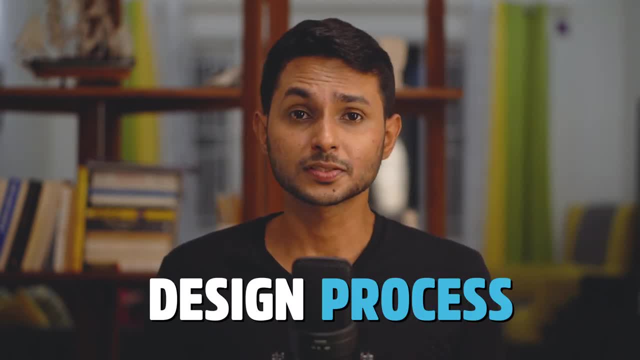 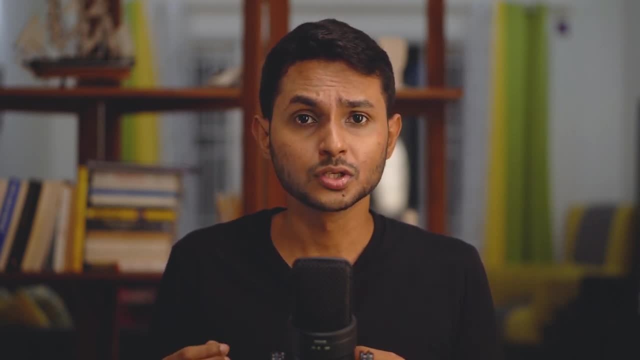 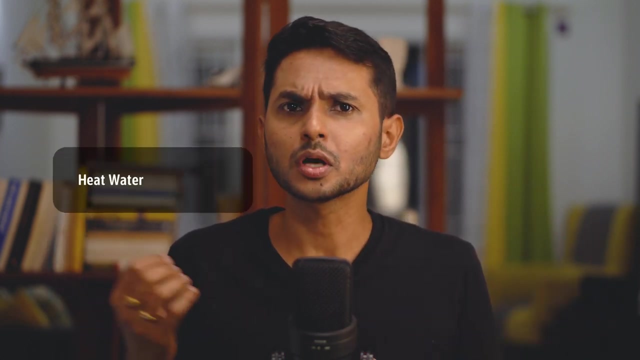 manageable channel. Before we go towards design process, let's try and understand what process means In simple words. process is a series of actions taken to achieve a particular end. Process can be made for anything- Making tea, for instance: Heat some water, add sugar and tea leaves. 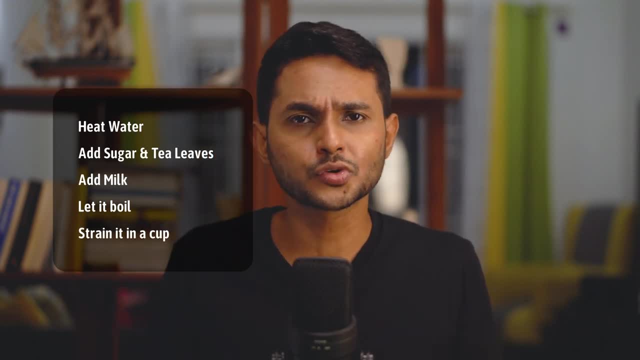 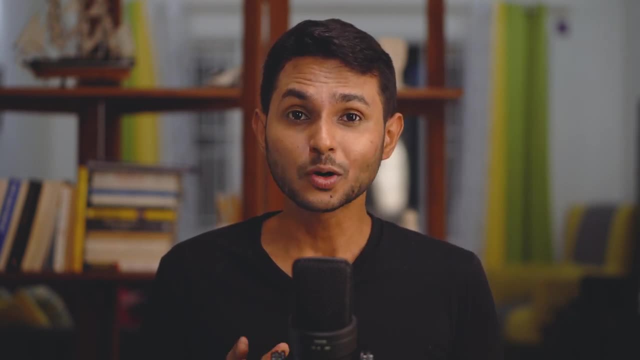 add some milk, boil it, strain it using a strainer And voila, your tea is ready. It's so simple when we follow step by step. But is that the only way to make tea? Well, it may seem like, because most of the people like 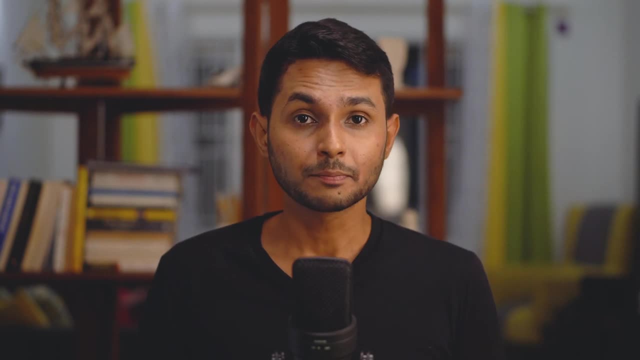 tea in that way, but not always. For example, I don't like milk in my tea and I prefer stevia over sugar. But milk and sugar are part of the process. Does it mean the process is wrong? Not really. It just means that mine is a special case. 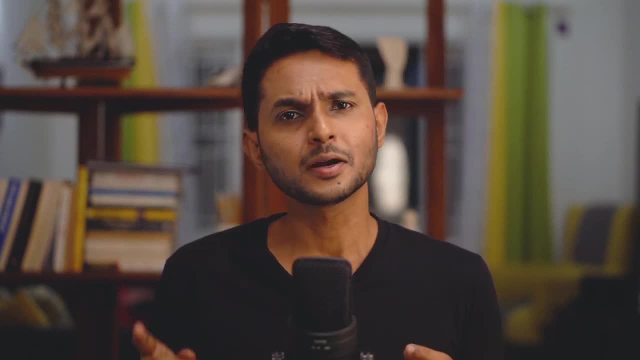 So what do I do? I just skip milk and I replace sugar with stevia, because both of them are sweeteners. I also reduce the quantity of leaves a bit just to balance the absence of milk, Otherwise it'll taste too bitter. The rest of the process just works fine. 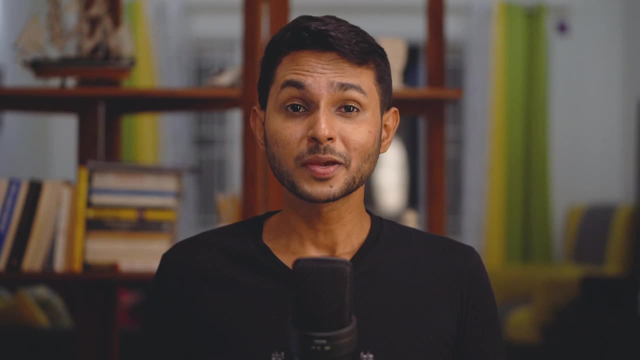 You see how easily I could modify the process. It's because I know exactly what each step does. If I had not known what each ingredient did and how it impacted other ingredients, I could have never made this modification. So a process is nothing but a set of things which works most of the time. 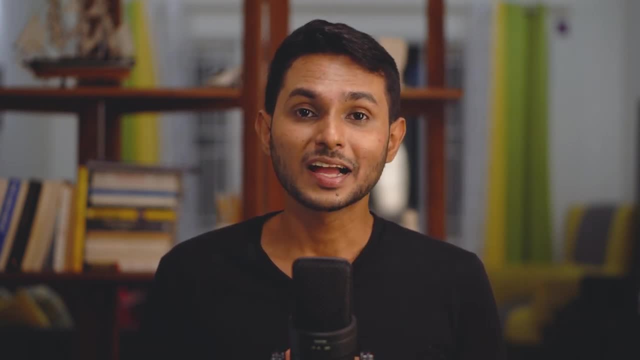 maybe 80-90% of the time. Some smart guy would have figured this out and published it as a source of truth called process, so that the not-so-smart-people can follow it to get their work done. This is the case with any formula or any process that you might've come in your life. 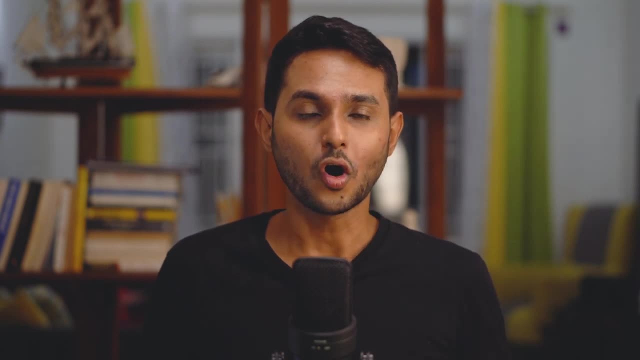 including the scary ones from math. So all set to apply the formula. But here's the catch, Of course I know I didn't do the math for a week. It's all good. As a result, because I've been doing it a few times, I've lost my temper. 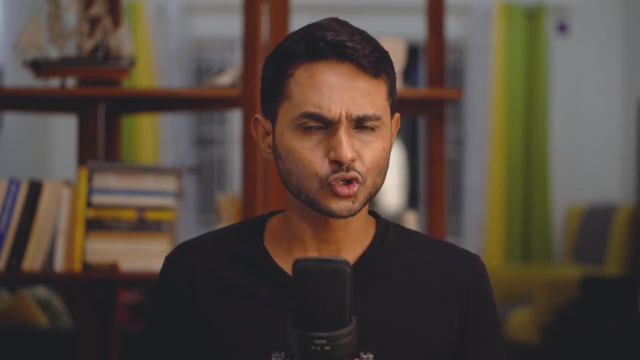 As a designer, you cannot afford to be that not-so-smart guy who blindly follows the formula or the process. I mean, come on, you are smart, And before you adopt or build a process for your design, you must understand what each and every step means. Only then you'll be able to make. 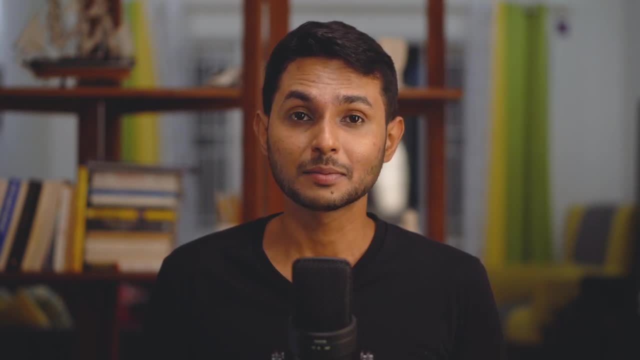 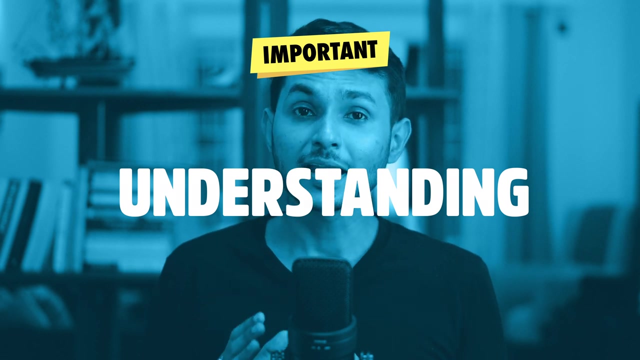 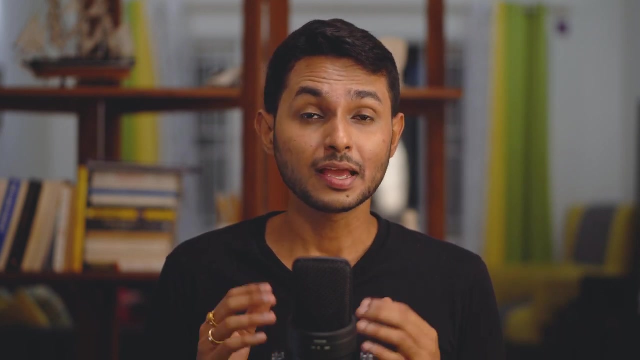 modifications to it as and when needed. Like someone has rightly said, first principles never fail. So here, my friends, the most important step in any design process is understanding, Understanding what the user wants and understanding what you can do for them. Remember, in this stage, everything that you can know, you must know. Like I said before, 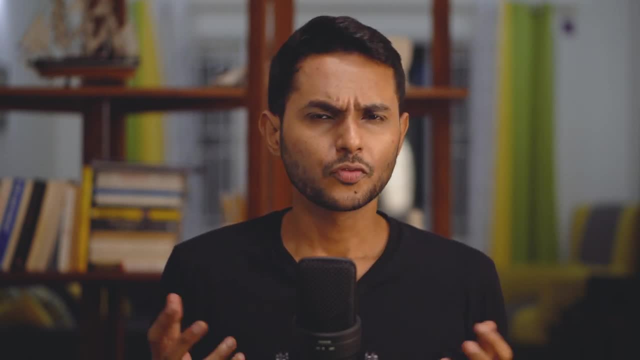 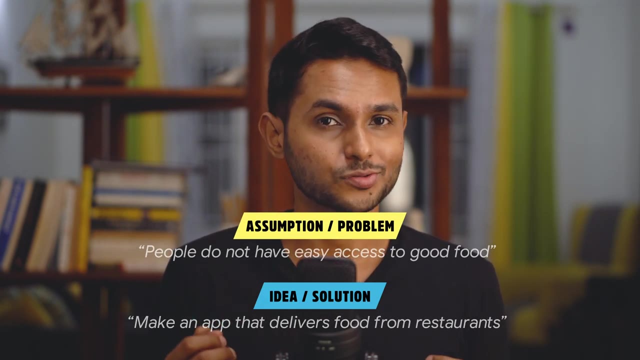 we often start with an idea and some assumptions around it. For example, one assumption could be: people don't have the right understanding of their design process, And so if you don't access to good food, It'll be nice to have an app that delivers food from restaurants. 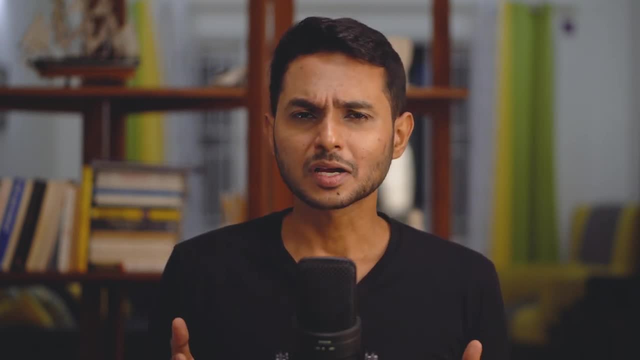 Now, this is a hypothesis. Most of the times our hypothesis can be right because we are experts in our respective fields and also we might have looked into a lot of data and all before arriving at the initial idea. But at times it can go terribly wrong as well. Let me tell you how bad 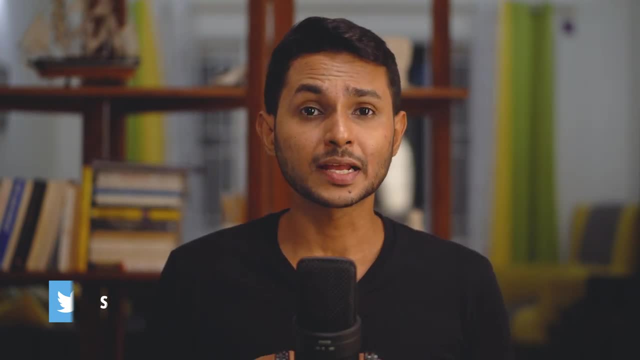 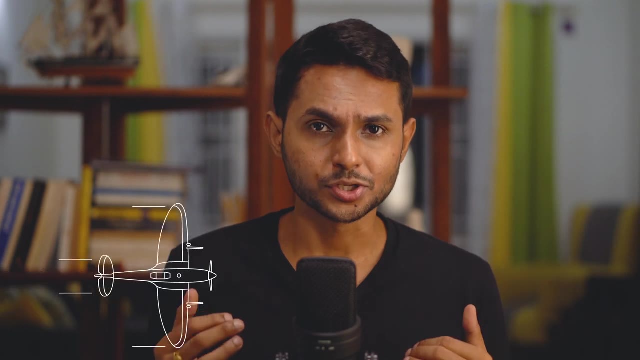 it can go. During World War II the British Air Force had lost a lot of planes to the anti-aircraft guns. So as a retrospection they inspected all the planes that came back from mission and they figured out that most of the planes had bullet marks on their wings. So obviously they 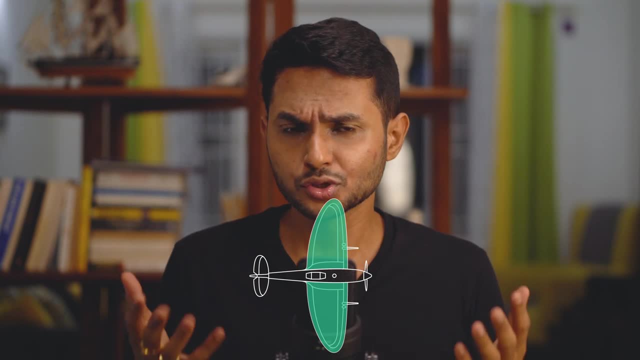 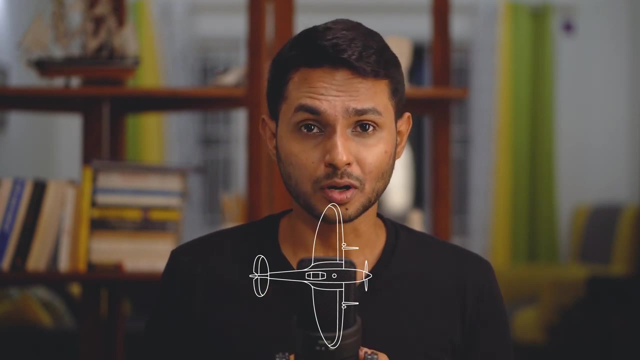 felt that adding an extra layer of protective armor around the wings should solve the problem. That was their hypothesis. When they delved deeper into the problem, they figured out that most of the planes that came back from mission had bullet marks on their wings. Most of the planes were, in fact, shot on the fuselage. And those planes never made it back because they would be destroyed instantly. So it made a lot more sense to armor the fuselage instead of the wings. If they had gone ahead and armored the wings, as per their initial hypothesis, they wouldn't have solved the complete problem. 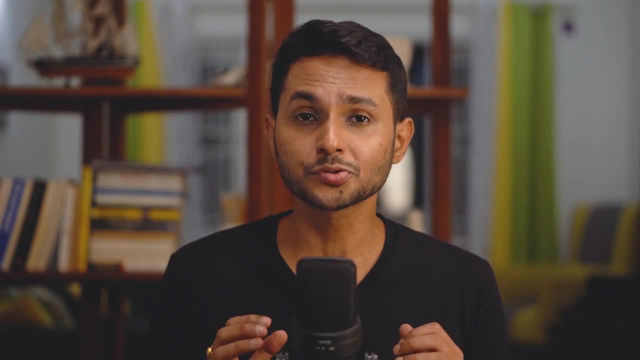 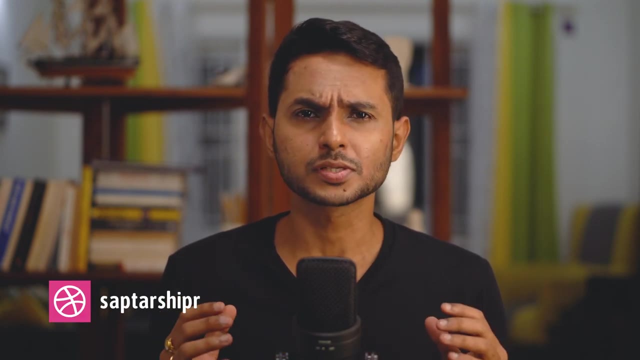 Hence this stage of understanding is super important and we should try and validate all our hypothesis in this. In a digital context, it may involve hours of internet browsing: reading about the industry, the problem, speaking to potential users, brainstorming the idea with a friend. 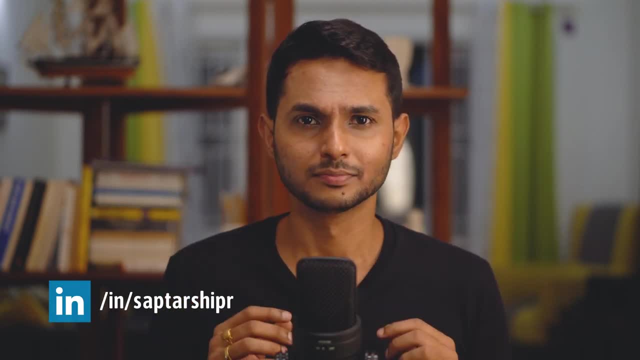 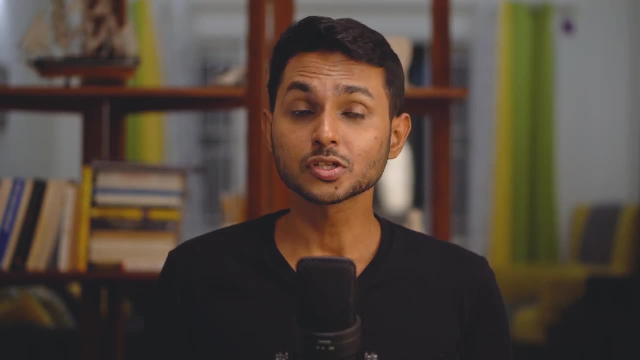 or even sitting alone and thinking about it in your head. If your mental canvas isn't big enough to hold your imagination, feel free to use paper and pen. This is also a good time to find out if you have any existing competition in the market. 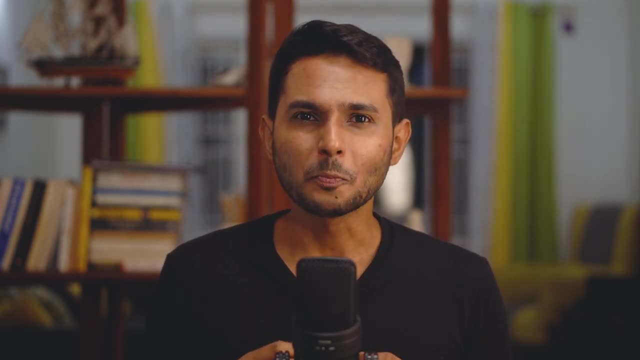 If you do try out their product. Check out what good or bad things their users are saying in social media and play store and app store reviews. If possible, speak to some of those users. Also, try and find out if there were other companies and players in the past who tried to do the same thing. 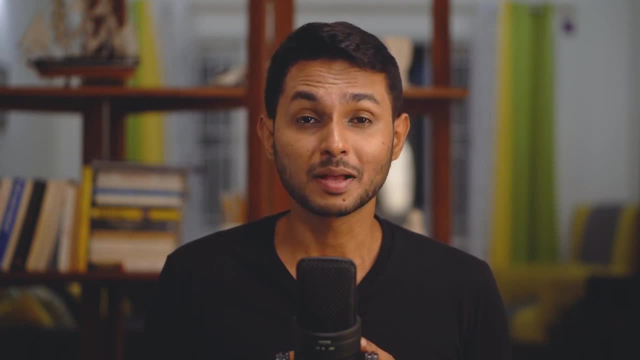 Find out why they had to shut down or why they failed. Remember, life is too short to learn from our own mistakes. We must learn from the mistakes as well as achievements of others. Once you have done this, you'll have a fair idea of 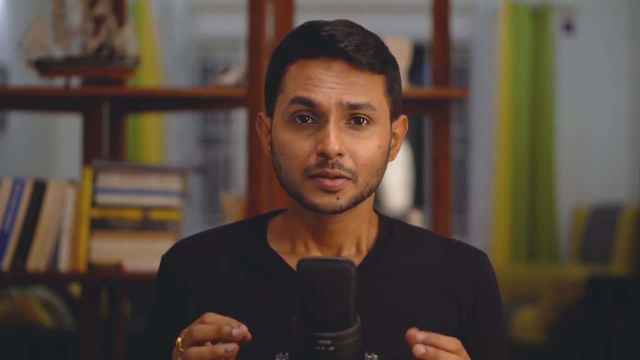 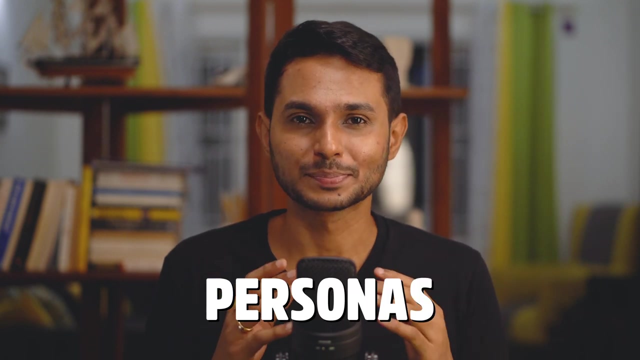 the kind of users your product should be targeted to: Try and create profiles of fictional characters based on them, with the details of who they are, what their primary goal is and what is the main barrier that stops them from achieving that goal. These characters are also called personas. 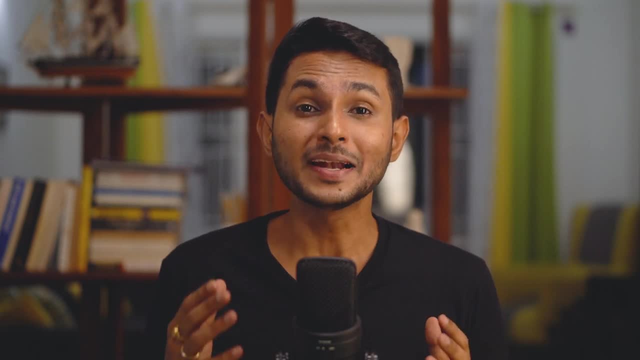 For projects that go on for a longer time. many designers prefer printing these profiles out on sheets of paper and sticking them around so that it's easier to refer to them. often, Once you go through this stage, you shouldn't have thoughts like: oh, I haven't thought what will happen when User A does X and Y in Scenario Z. 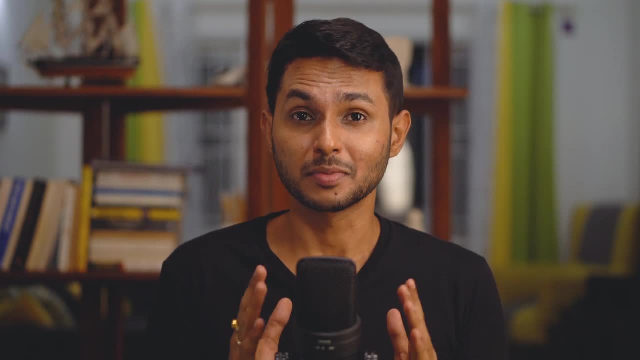 Make sure you understand every nitty-gritty associated with their premise. Many people also refer to this stage as research, But I won't suggest that, because research is only a means and not the end goal of this stage. In case of tea, the point was to sweeten it. 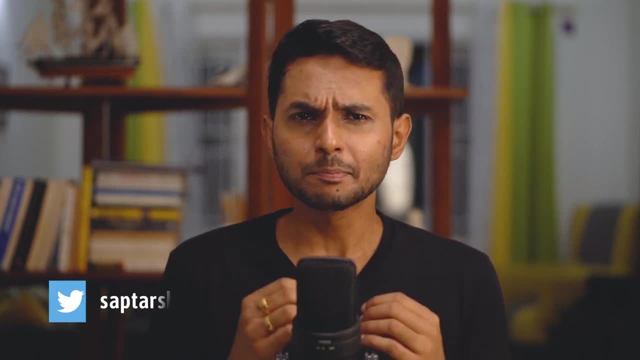 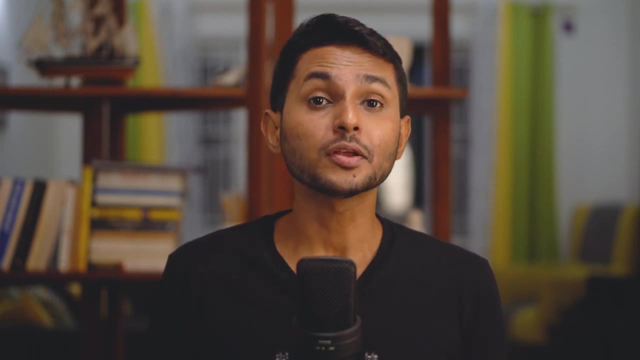 And whether I use sugar, jaggery, stevia or choose completely to skip it depended on the situation and the preference of the consumer. In the same way, the point of this stage is to understand the problem completely. Whether you do your own research, use the findings from an existing research. 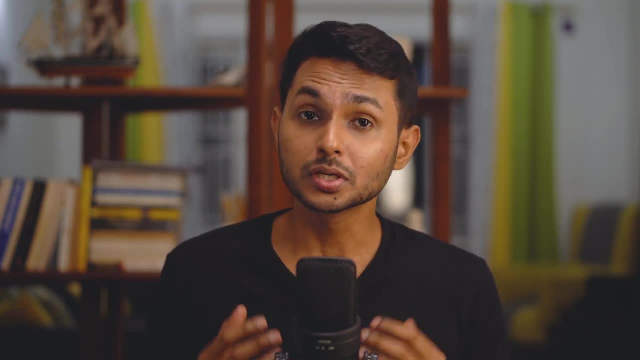 or follow a mix of both. again, completely depends on the situation At times, if you feel you naturally have all the context that is needed, all the understanding that is needed, then you may choose to skip this step. Yes, you heard me, right. 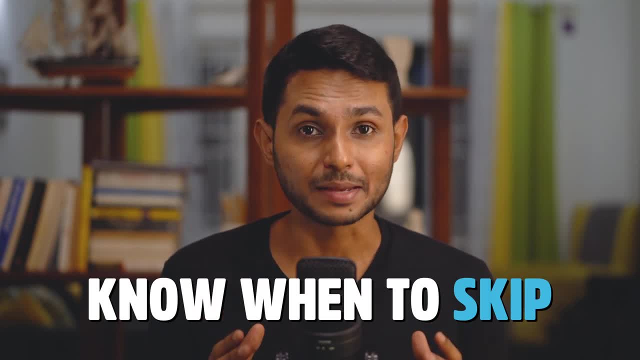 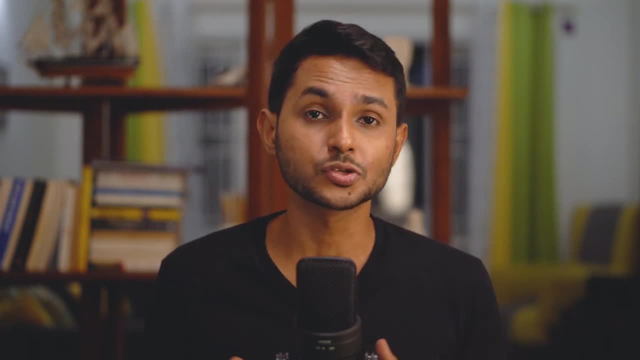 I just said, you can completely skip the most important step. This happens in case of smaller projects, like incremental changes, where you already have all the context, since you have been working on it for quite some time. After you do all these things, you will have a revised idea and approach.